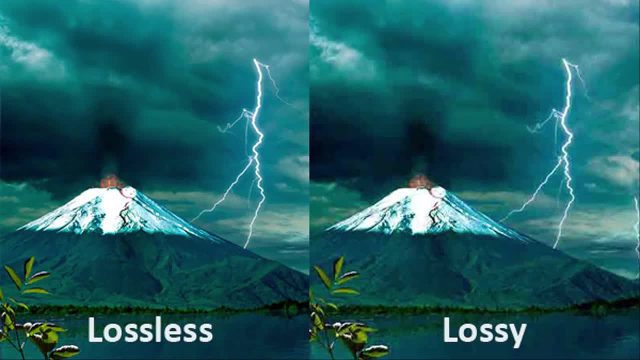 in a more efficient way, And it would need to ultimately be run through a decompression algorithm on the receiving computer's end to get that original file back exactly the way it was, Whereas lossy compression is actually sacrificing some information about a file. So in this example, 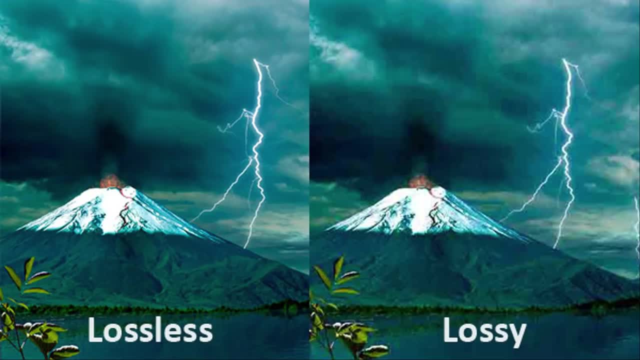 that I've got here. the lossless image on the left probably looks pretty much the same way that it would on the raw data that was taken by the camera, Whereas the lossless image on the left probably looks pretty much the same way that it would on the raw data that was taken by the camera. 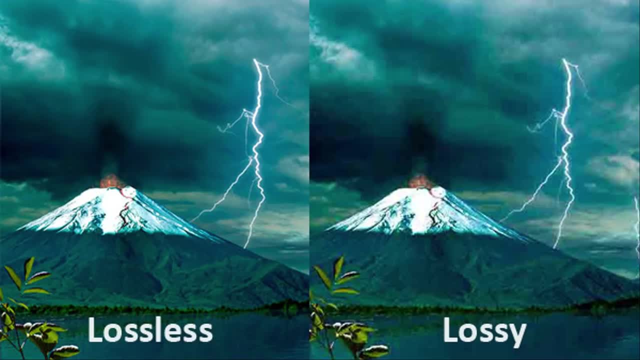 lossless one. clearly, there's some information lost. there's quite a degradation in quality. it's a lot blockier, a lot more pixelated, and this is basically because you've got pixel areas here that are just being summarized to one or two colors instead of being many different colors. 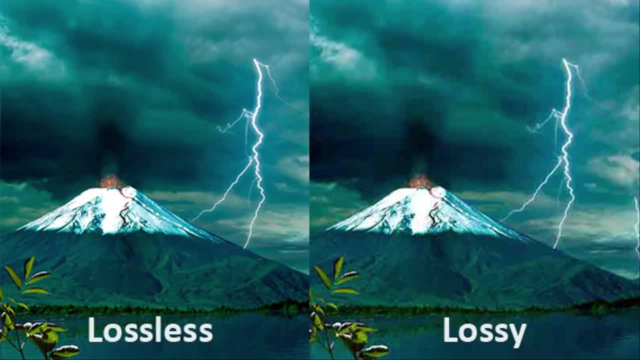 like we see on the left hand side. so a lot of information is sacrificed and typically with these lossy compressions they don't need to be run through decompression on the original machine to rearrange things, because they're not just rearranging the data, they're actually. 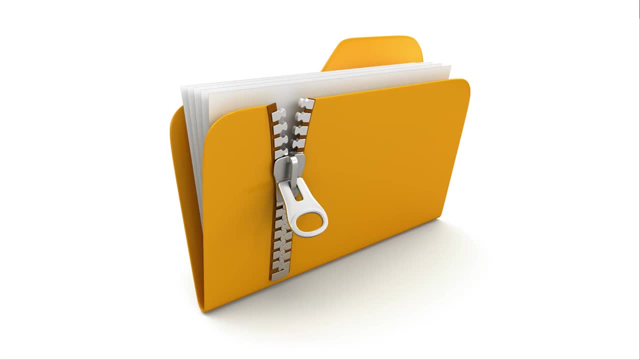 removing some data, so lossless encryption or lossless compression. rather, this is what you would use in the case of downloading really large files like a zip, a tar archive or a cab file, because you can imagine, if this is some code that you need to compile, it can't be using a. 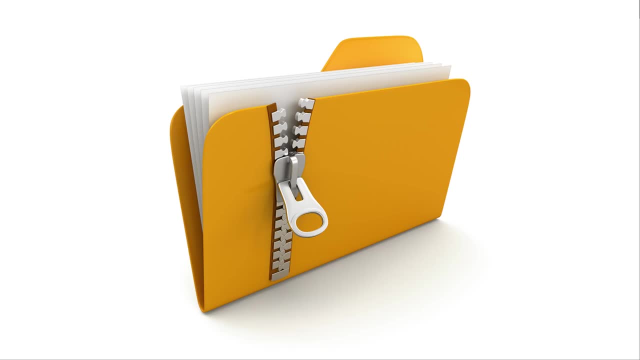 lossy compression. if something's actually missing from the code, you're going to get an error when you go to compile it. so essentially, what you're doing with this is you're saving bandwidth by transferring a smaller file across the wire at the cost of cpu power to actually open up and do that decompression of the zip or the archive on the receiving machine. but this makes a lot of sense to do because cpu power is generally much more abundant and much cheaper than network death neglect, because you use cpu power to actually sort of lower the desired bandwidth. 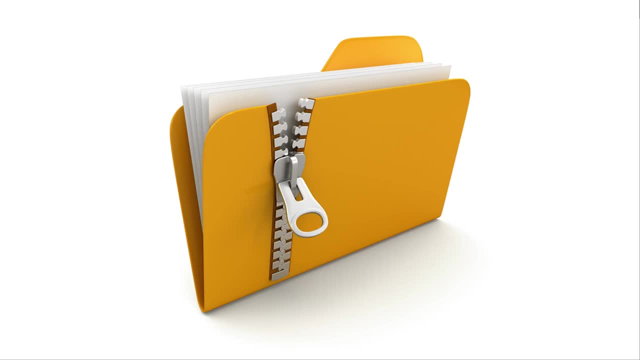 mma and lower the listener speed. so with open, worthy, comp pulsing programs you can do a lot simple things like reduce that stated latency time, move around in time a lot of the time and say you know what this button boyfriend should be serving better than jfd. so then, 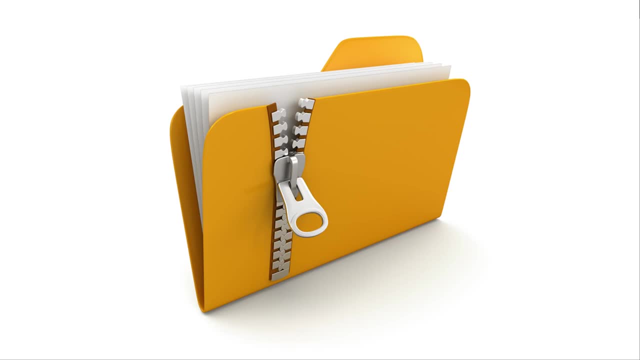 a lot of the more complex things that the open kunna and myths are involved inraj Galaxy would be more shortened and of course, that would say more stringent orderedös that we'd only get by making a fewNo remember, just go back in to the pre-production during every file that you've done. 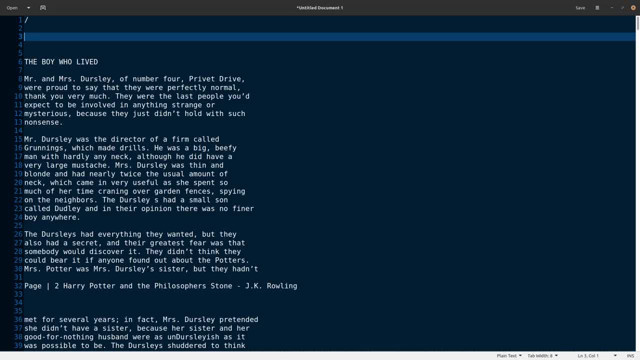 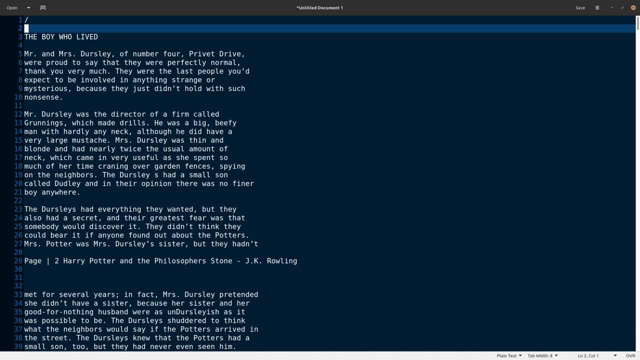 things. So the best way to show this would probably be in a text file. This is actually the text of the first Harry Potter book, So to compress it, there's a few things that we can do. One: we can just get rid of, you know, any blank spaces or any blank lines, so that we're not using 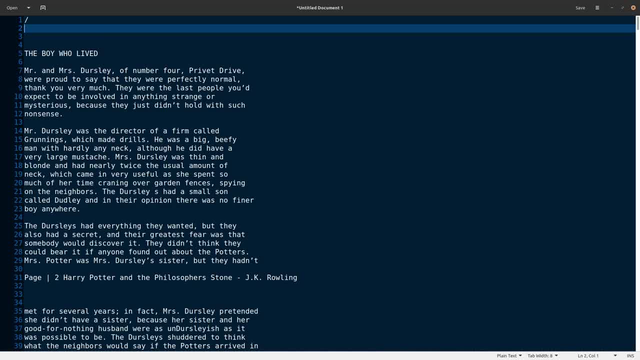 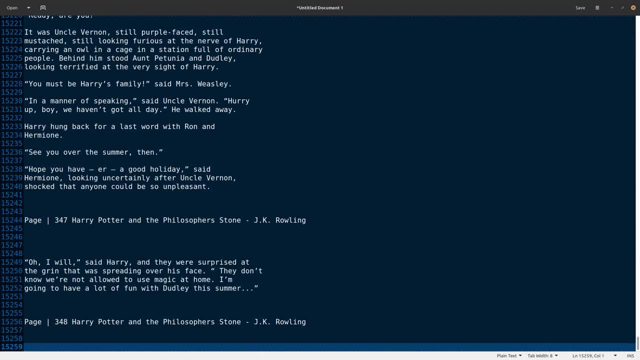 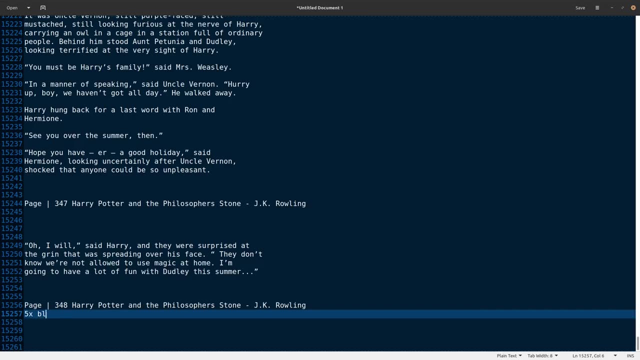 up any data with that. What we would really want to do is just create summaries of it. So instead of like whoops, didn't mean to delete everything there, Instead of having, like you know, three or four or five blank lines here, we might just say like 5x blank or something else that is shorter. 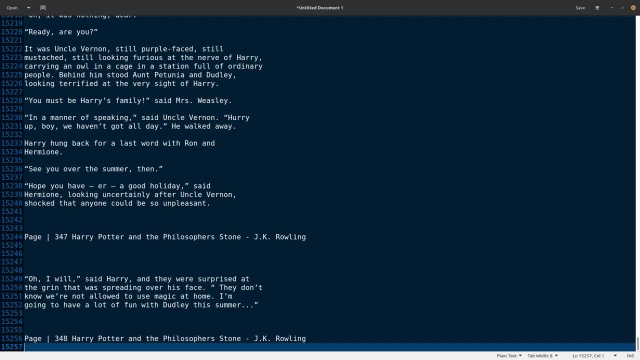 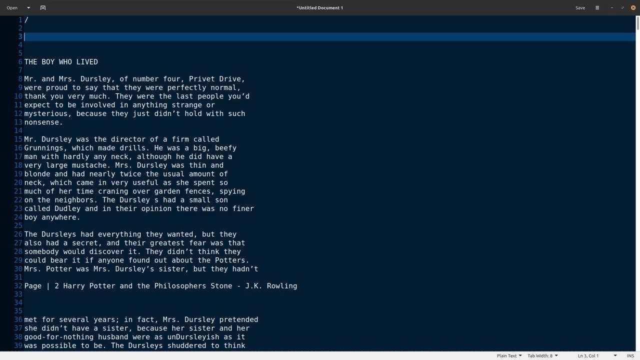 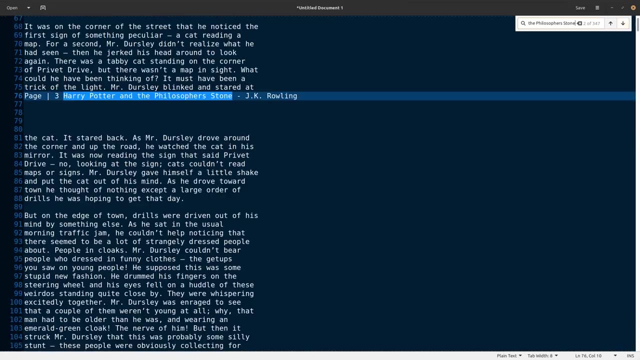 code for that and then just delete all of those blank lines. Another thing that we'd want to do is, like I said, summarize any repeated data. So this phrase here- Harry Potter and the Philosopher's Stone- is very common. If we search for it, it appears 347 times, because basically this appears every time you're. 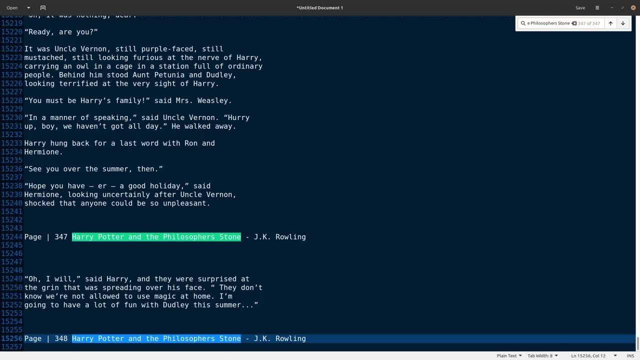 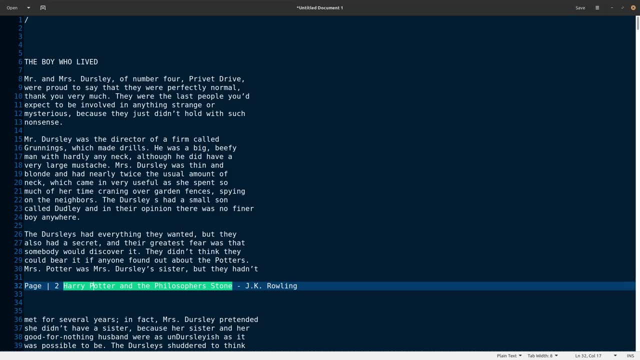 technically going to another page. So this shows up a whole lot and it uses a lot of bytes to repeat that every single time. So what I would want to do is delete all occurrences of this and just have it one time up here at the top of the file. 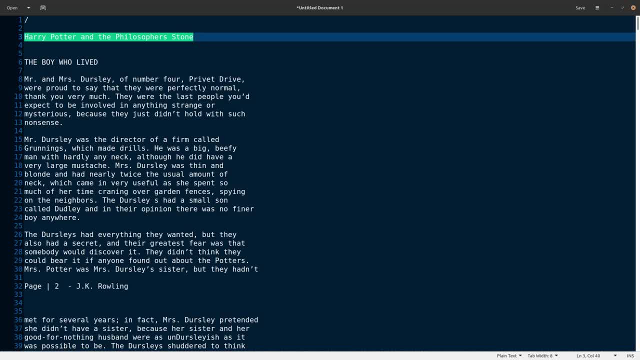 So this is basically the first time that we've done that, So we're going to do that. This is about 40 bytes or so, And then we need to provide some information about where to reinsert the text for that decompression algorithm. So we know that that's going to appear on line 33. 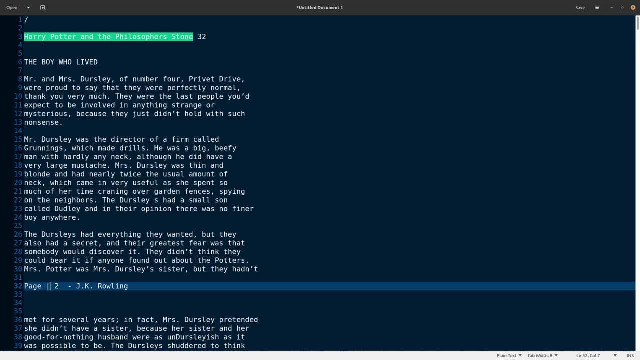 or 32, rather, And let's see how many characters over it is. So 1, 2, 3, 4, 5, 6.. We'll say it's 7 characters over. So that's the coordinates for where this data is going to go, And then you would. 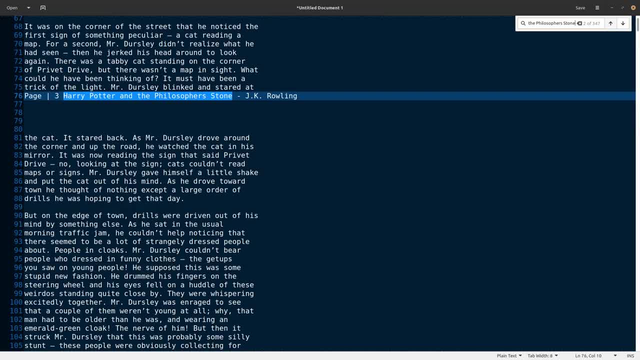 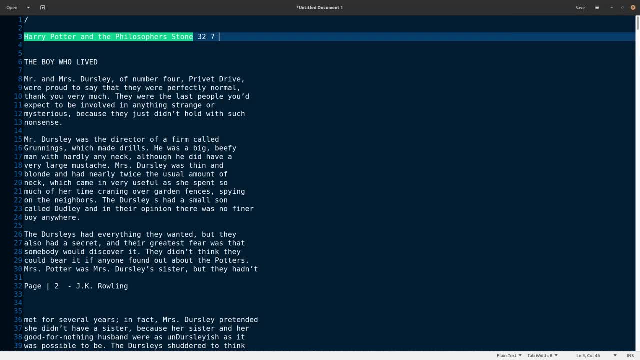 just repeat that over and over and over again. So like the next occurrence is on 76. And we'll say it's again 10 over 2 the right, So we'll say 76,, 10.. And these coordinates obviously use way less. 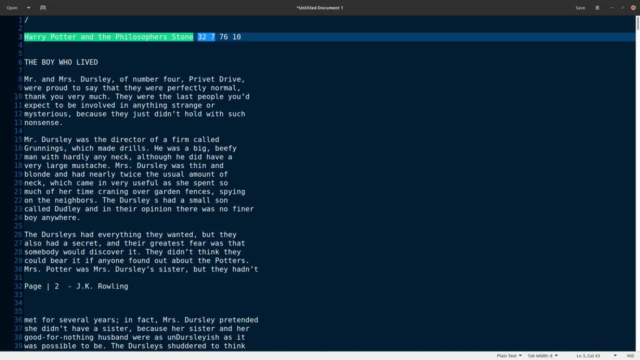 data than writing out this whole phrase. You know these are using up maybe- well, not even 10 bytes of data, but we'll say 10 just to make it make the math simpler. And this is using roughly 40. So we're saving 30 bytes of data every single time we add another coordinate. So you repeat. 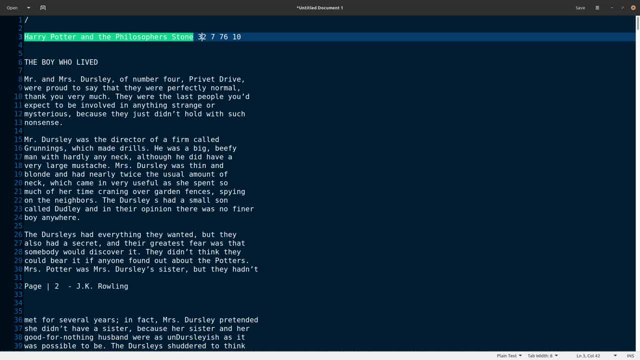 this process for all of the phrases or words that appear, a lot things like main characters names and so on, And suddenly you have a long list of words at the top of the file and their coordinates, and then some garbled English at the bottom of just you know unique text where those 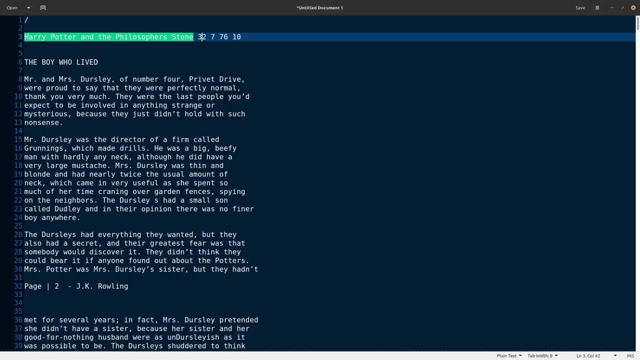 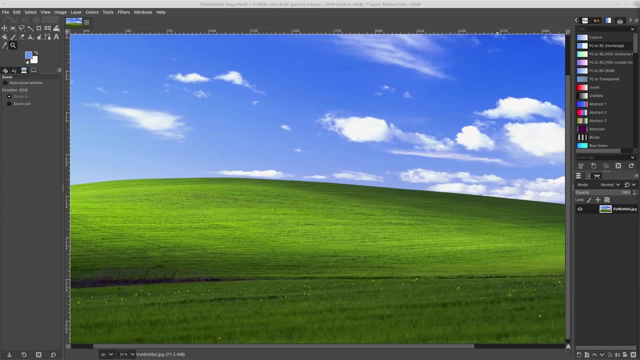 words were removed from, And what you would get is a file that is smaller than the original, but it contains everything that the end computer needs to then reassemble the file into a sensible work that you can read. The same idea can be applied to pictures, So take this image for. 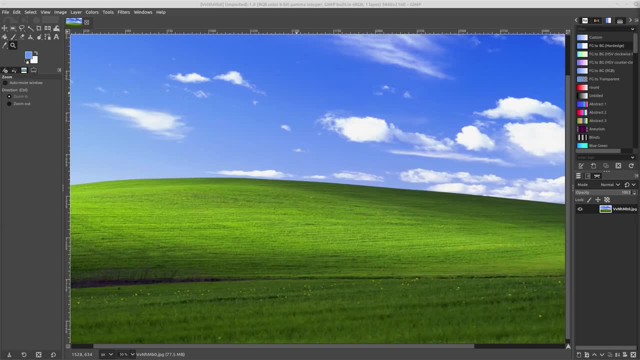 example. This is Windows XP Bliss. This image has probably been seen by more people than any other in history. Think about that for a moment. It's also a very simple picture because it's really just a big field with some rolling hills and you've got a blue sky. 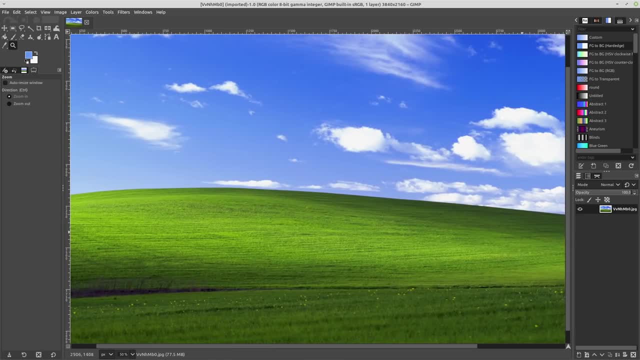 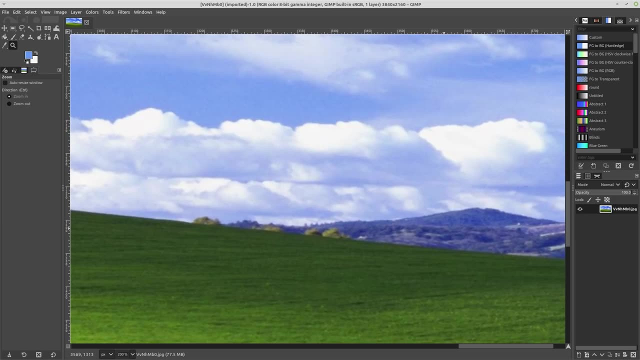 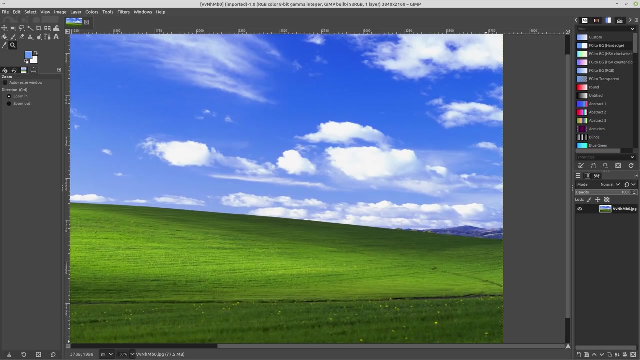 background with some white clouds, and way off here over to the right you've got, like, some mountains or some other hills that don't really have a lot of information anyway, because it's such a small part of the picture. It's basically just sort of a bluish, grayish clump of pixels. 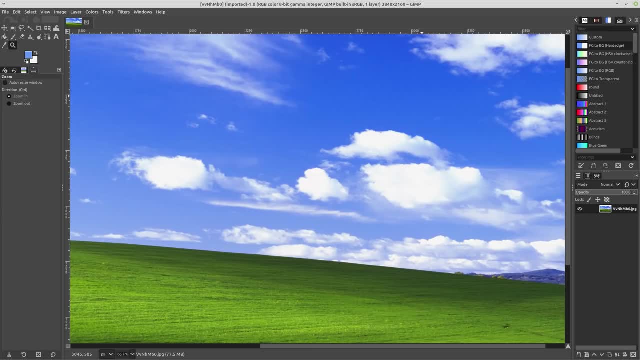 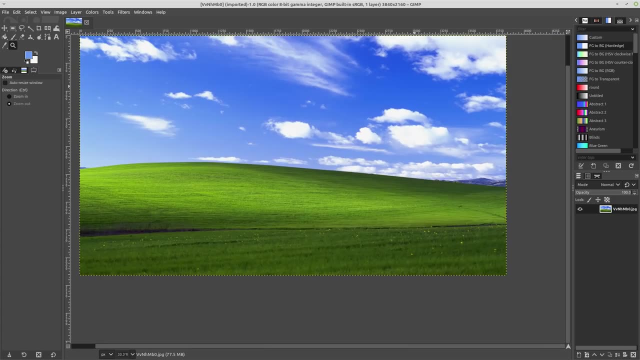 So the individual pixels that make up this picture. they've got to be fairly similar, especially in spots like this. In fact, if you made up a list of all of the colors that are used in this entire picture and you wrote out all of their hex values, you might only have a few hundred or a few thousand. 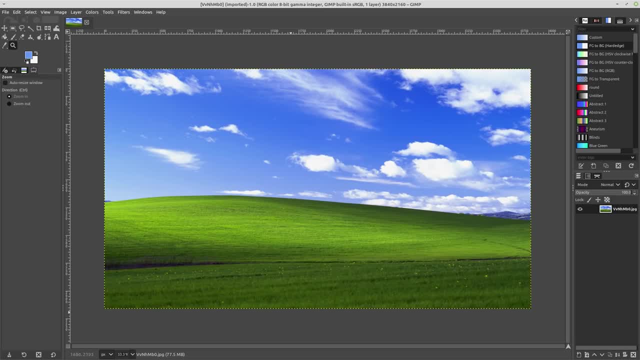 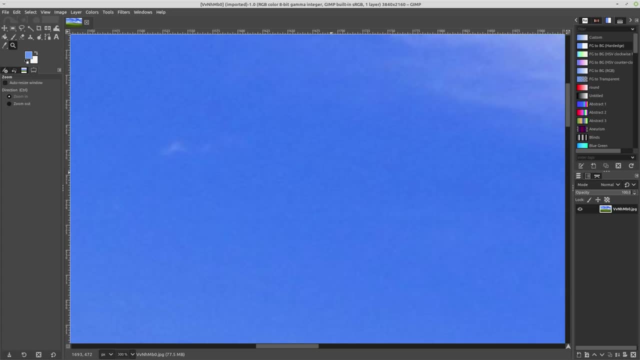 different colors. So, just like how we shortened our text files, we might say that, like you know, this area of blue right here is all the same color. We're going to say it's all one hex value blue. and then, you know, this area here is another hex value of blue. Now, this could end up being: 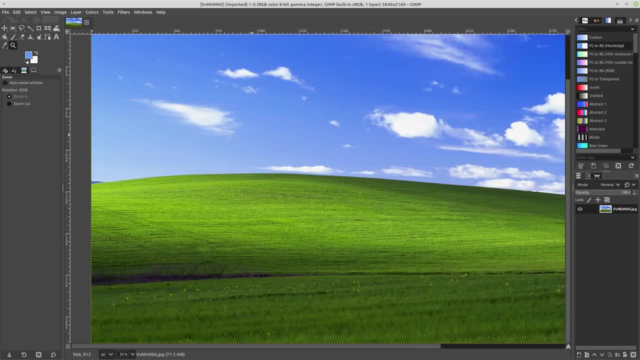 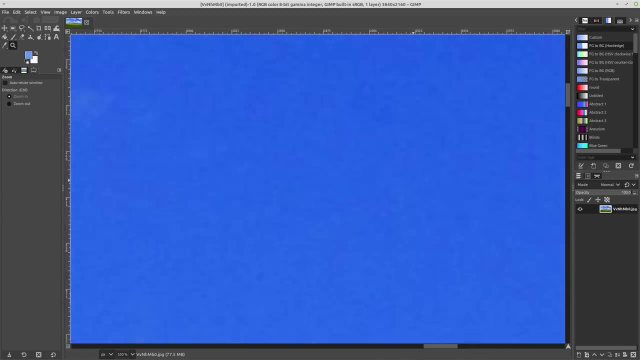 a lossy compression. In fact, all of these pixels are not exactly the same color like, even if we zoom in where it looks about the same, like maybe here, this all pretty much looks the same, but once we get in really far we can see that it isn't exactly the same. Where's my color picker tool? 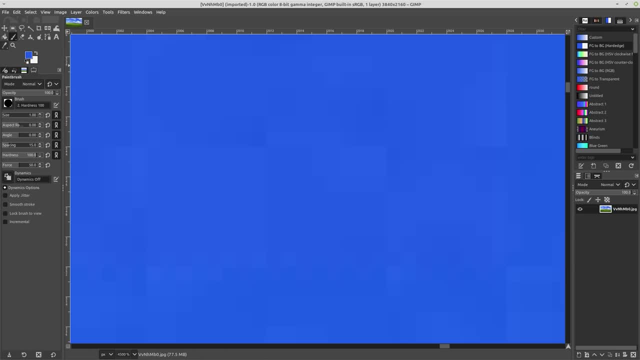 And I need to. so if I go on to this pixel and I open up the color information so you can see there is some slight variation in the different pixels here. but when you're zoomed out, especially on an image like this, because this is actually a 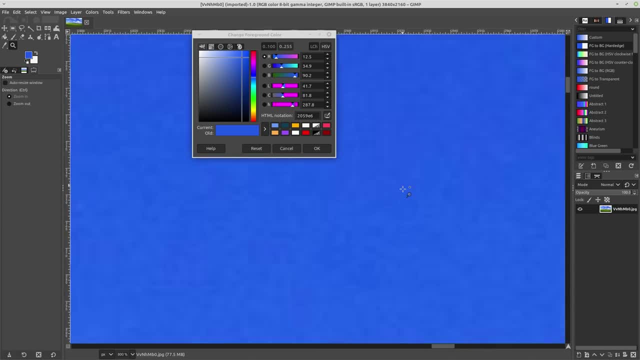 4k version of Bliss. you can change it and you wouldn't really notice. So like, let's, let's do this, let's change. oh, these two right next to each other actually are the same and this one here, but that's just because it's upscaled. Alright, so let's change. 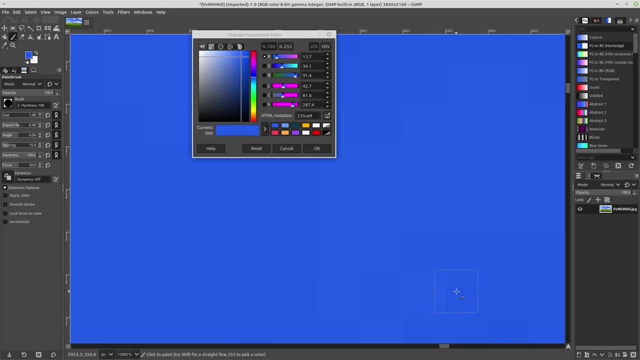 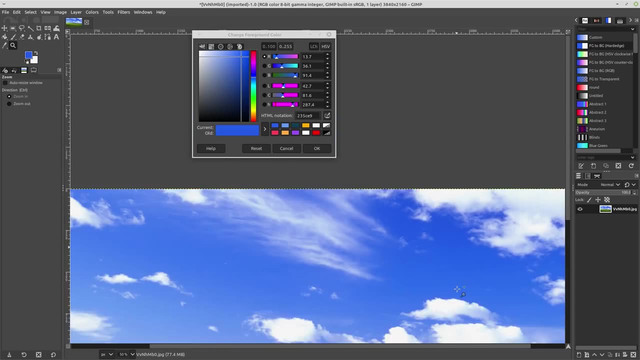 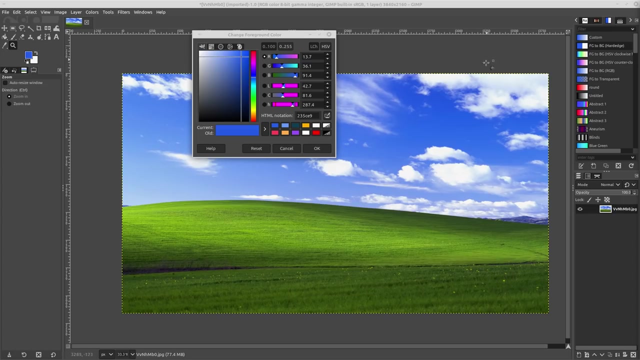 this. it will change that one here, that one here, so you can see it when it's zoomed in a lot. but if we zoom out, naked eye wouldn't really notice that. Now the more common type of image compression, such as P and J or P and G to JPEG, 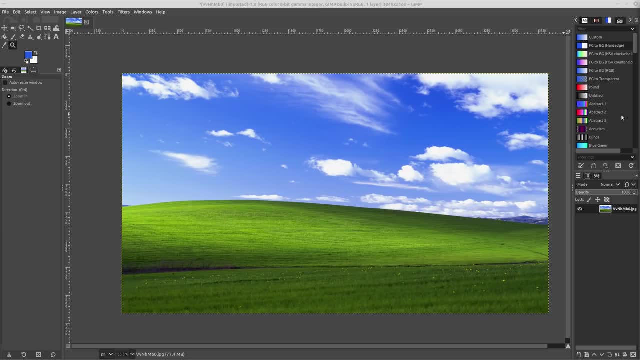 or especially RAW to JPEG. they're much more intelligent than this and they produce images that look almost identical. You're still losing some image data with RAW to JPEG, but what you're mostly losing is metadata, like you know, sensor information and all the rest of the XF data that provides information about the camera settings. 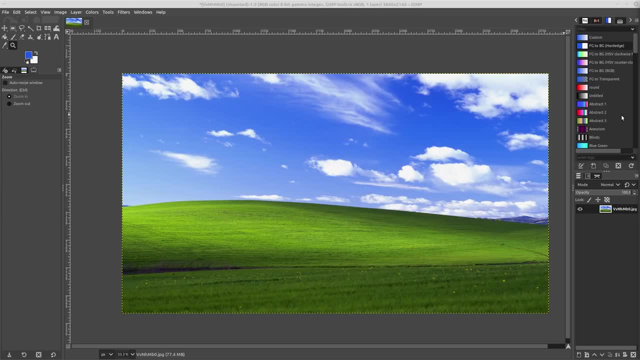 that were used during that shot. Now, that's very important if you're going to edit the file, but when you're just exporting it to show it to other people, It makes a lot more sense to have a file that's like five or ten times smaller, with details that most human beings probably won't really notice being gone from a RAW, compared to a JPEG.